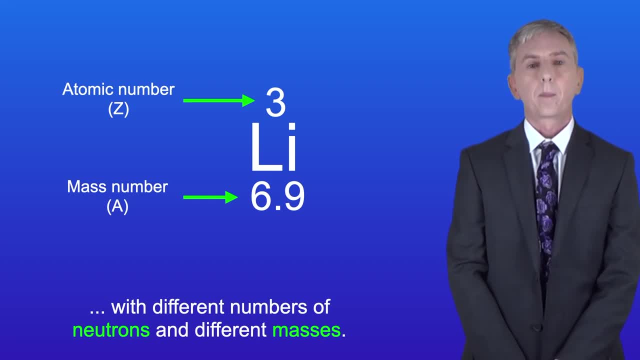 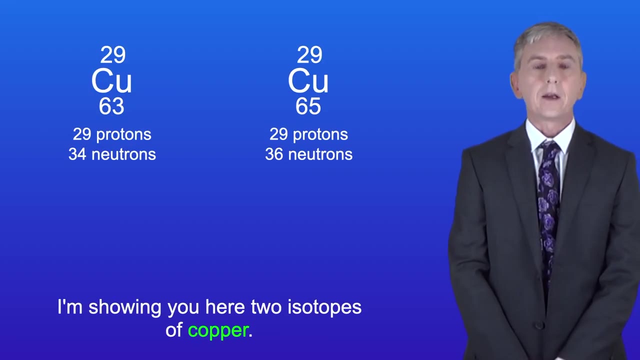 with different numbers of neutrons and different masses. Now that is a key definition and you could be asked it in your exam, so you need to learn it. All of the isotopes of an element react in the same way, and that's because they all have the same electron configuration. I'm showing you here two 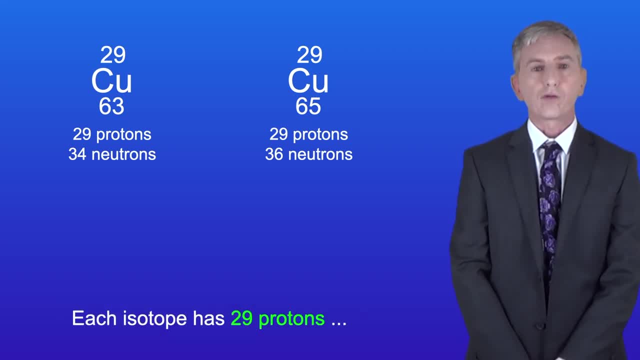 isotopes of copper. Each isotope has got 29 protons, but the number of neutrons varies. This isotope has 34 neutrons, but this isotope has 36 neutrons. Now, one key idea you need to understand is abundance. The abundance tells us how common each isotope is. Around 69% of copper atoms are. 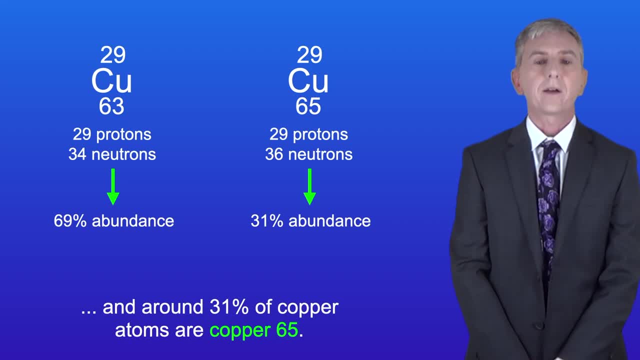 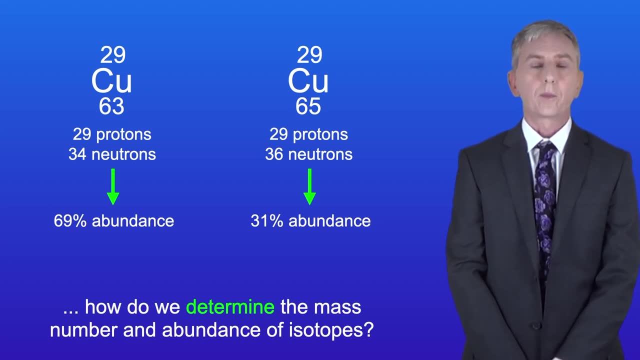 copper 63 and around 31% of copper atoms are copper 65. So the question is: how do we determine the mass number and abundance of isotopes? Well, to do that, we use a machine called a mass spectrometer, and you could be asked that in your exam. Now, if you're following the AQA, 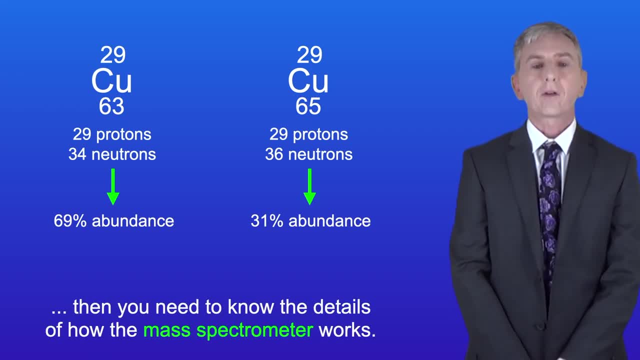 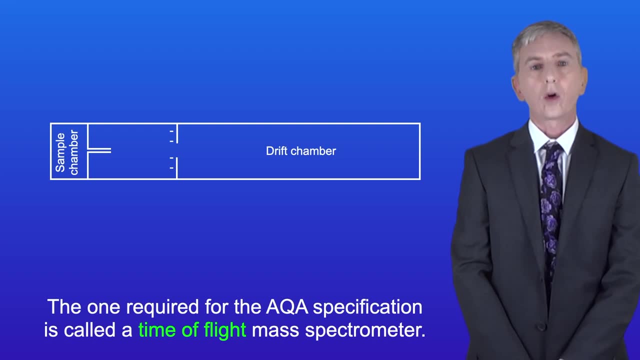 specification, then you need to know the details of how the mass spectrometer works. There are several different types of mass spectrometer, but the one required for the AQA specification is called a time-of-flight mass spectrometer. In the first stage, we take a sample of the element that we're 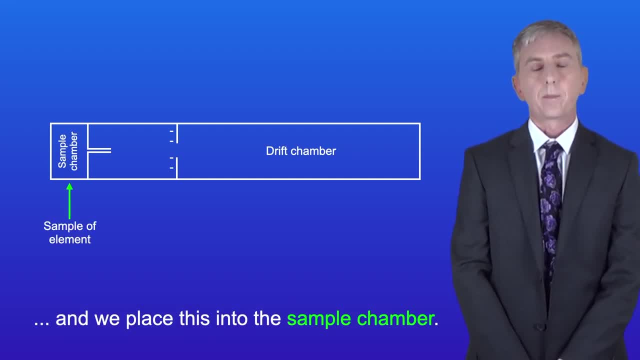 interested in and we place this into the spectrum. In the second stage, we take a sample of the element that we're interested in and we place this into the spectrum sample chamber. This sample contains all of the different isotopes of that element. The atoms then go through a process called ionization and this converts all of the atoms. 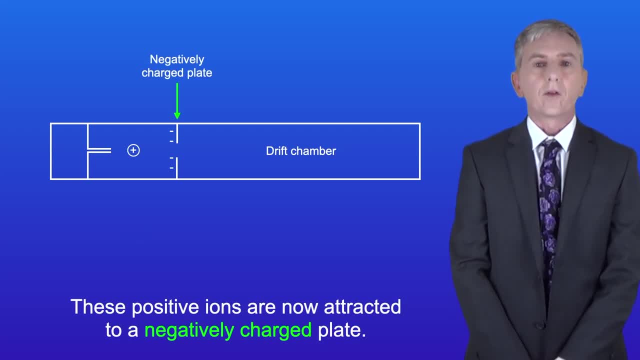 into positive ions. These positive ions are now attracted to a negatively charged plate. This negative charge causes the ions to accelerate and this increases the kinetic energy of the ions. Now, the key fact that you need to learn is that all of the ions with the same charge will have 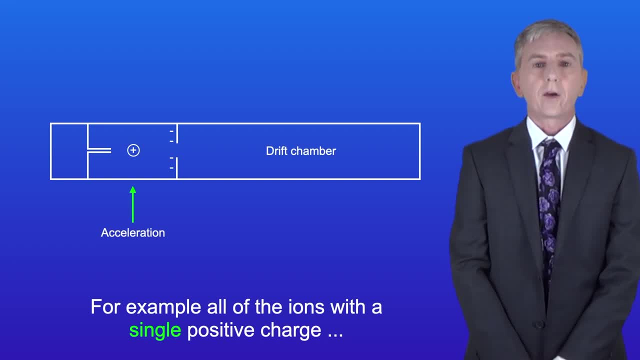 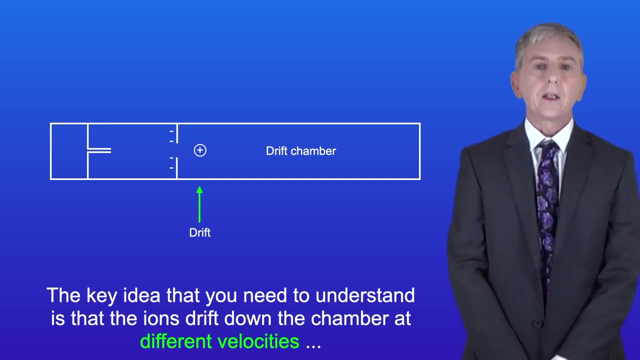 the same kinetic energy. For example, all of the ions with a single positive charge will have the same kinetic energy as each other. Once the ions pass through the negative plate, they stop accelerating and they drift down the chamber towards the detector. Now the key idea you need. 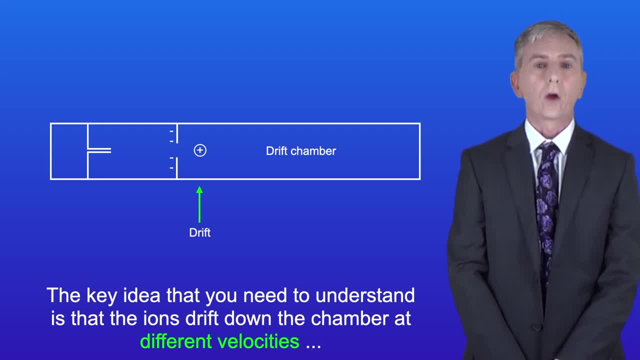 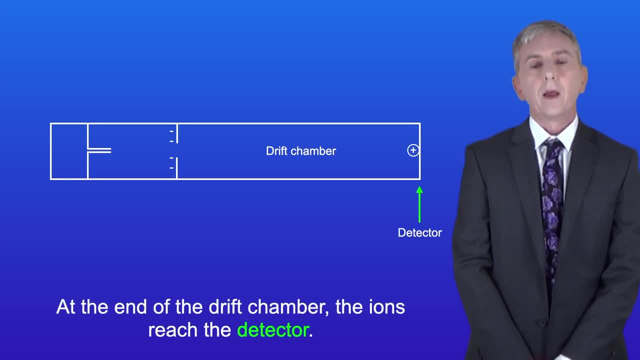 to understand is that the ions drift down the chamber at different velocities, with the lighter ions moving faster than the heavier ions. At the end of the drift chamber, the ions reach the detector. Now each positive ion gains electrons from the detector. So, for example, an ion with a single 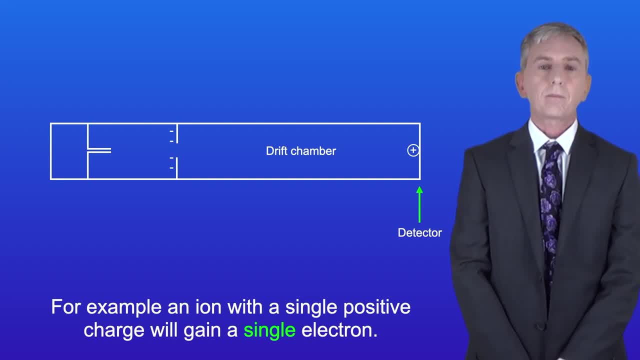 positive charge will gain a single electron. This transfer of electrons causes a current to flow. Imagine that we've got two different isotopes moving down the drift chamber. Ions of the lighter isotope will have a greater velocity and will reach the detector first. 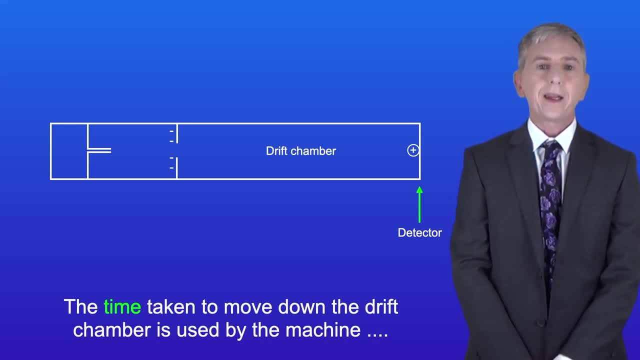 The time taken to move down the drift chamber is used by the machine to determine the mass of the and the size of the current produced when each isotope hits. the detector is used to determine the abundance of each isotope. A more abundant isotope will produce a greater current than a. 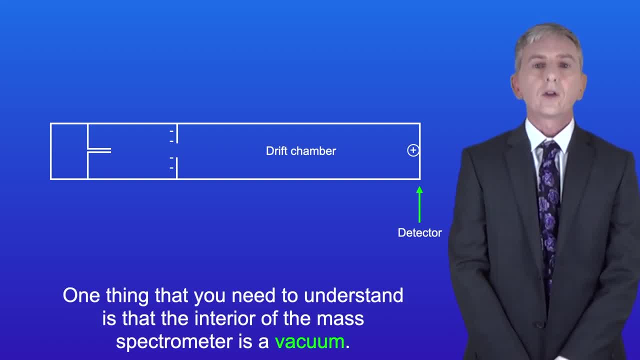 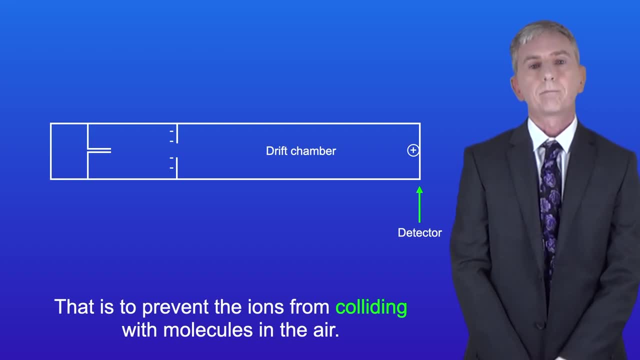 less abundant isotope. Now, one thing you need to understand is that the interior of the mass spectrometer is a vacuum, and that's to prevent the ions from colliding with molecules in the air Coming up. we're going to look at how to interpret a mass spectrum. 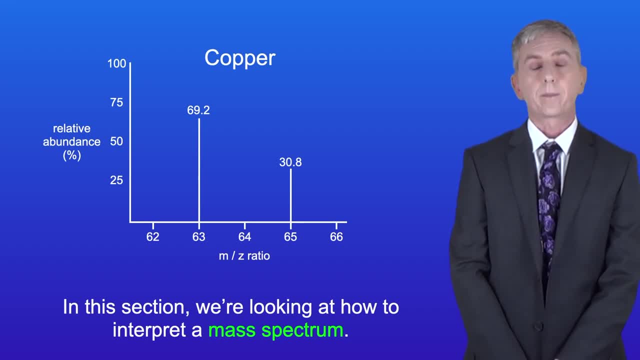 Okay. so in this section we're going to look at how to interpret a mass spectrum. I'm showing you here the mass spectrum for the element copper. The first thing to notice is that the spectrum has got two main peaks. This tells us that copper has two main isotopes. 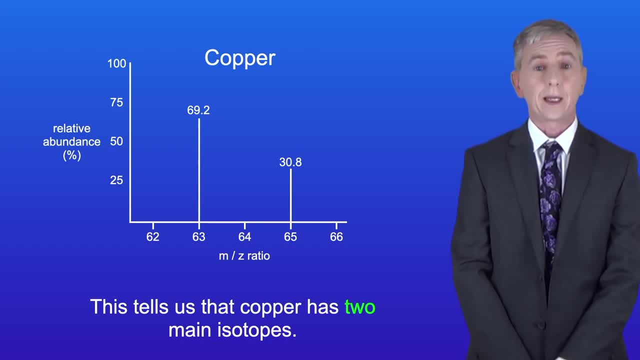 The y-axis shows us the relative abundance for the two isotopes. This is given as a percentage of the total and often these are shown at the top of each peak, like I'm showing you here. On the x-axis we've got the mz ratio. This is the ratio of the mass of each atom. 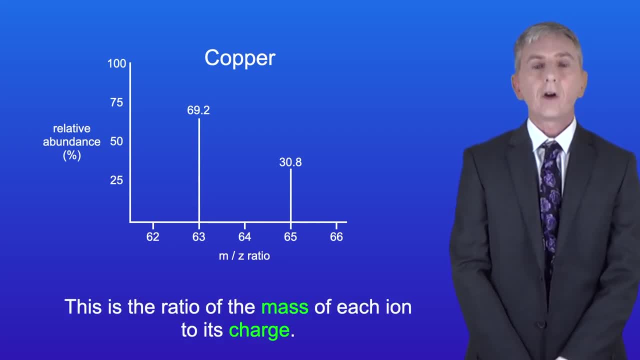 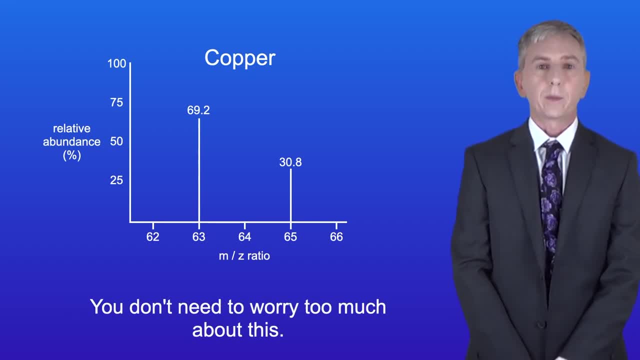 So if we look at the x-axis, we can see that the x-axis is the mass of the atom. So if we look at the x-axis, we can see that the x-axis is the mass of the atom. You don't need to worry too much about this. Almost all of the ions have a single positive. 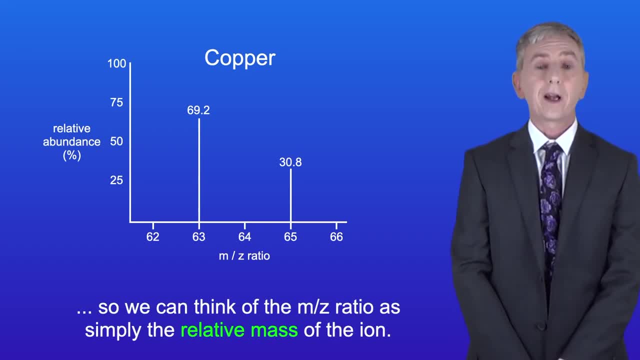 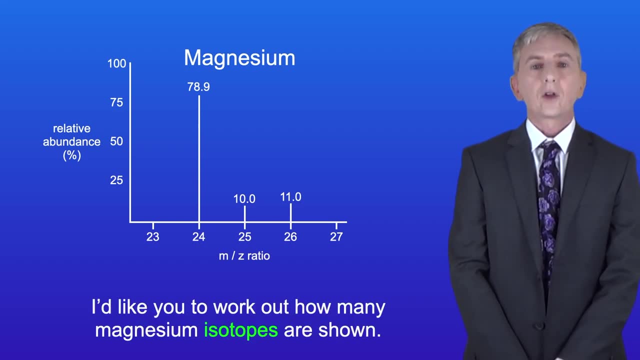 charge. So we can think of the mz ratio as simply the relative mass of the ion. Here's a mass spectrum for you to interpret. This is for the element magnesium. I'd like you to work out how many magnesium isotopes are shown.